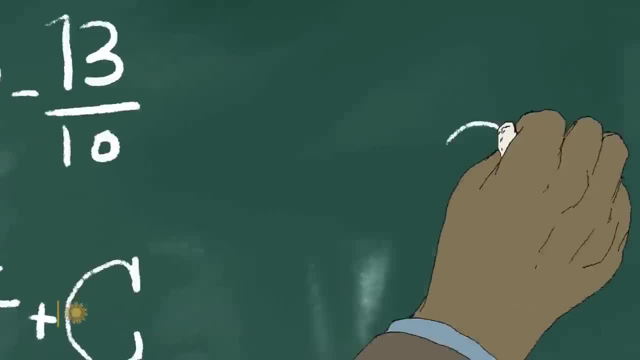 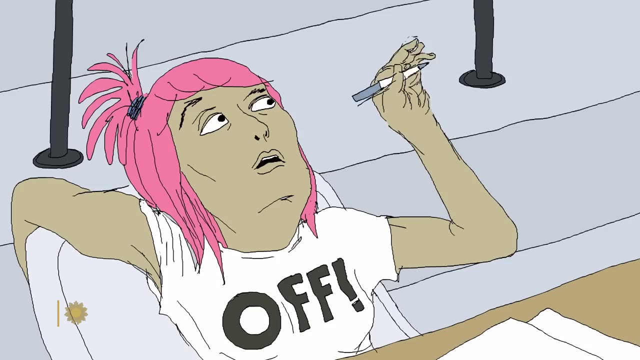 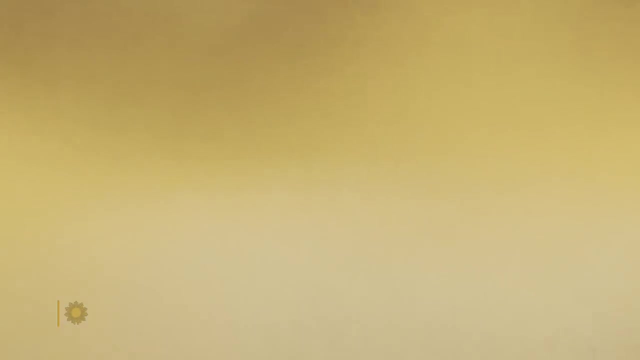 and I should tell you it's a pretty big number. it's two times 10 to the 23rd joules of heat energy per year, which, for those of you don't know what a jewel is, it's the equivalent of you've seen atomic bombs like the one in Hiroshima. that bomb, when it went off, gave off lots of. 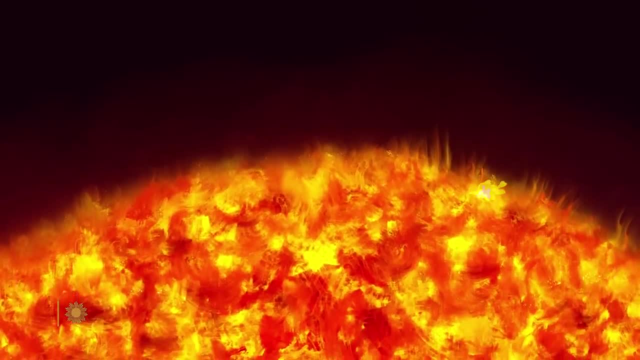 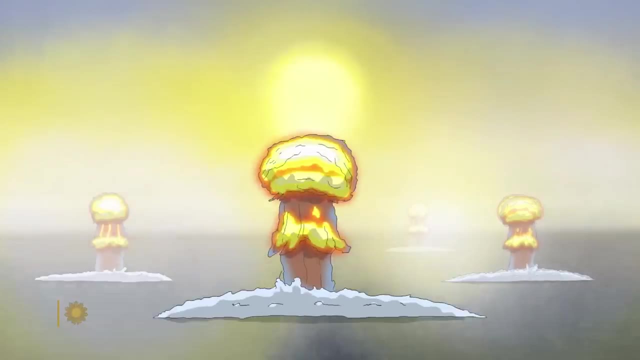 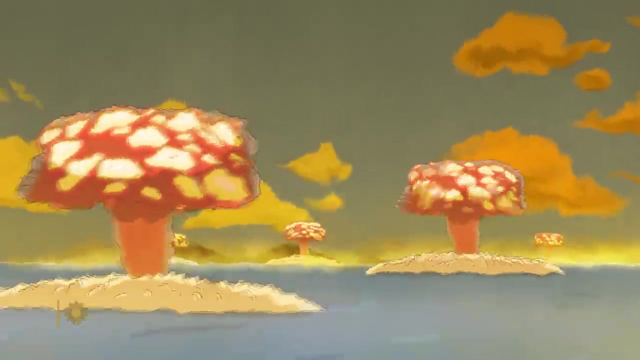 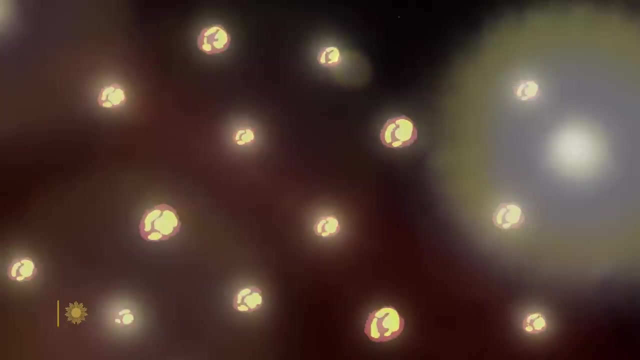 heat, very briefly hitting temperatures hot or hotter than the sun itself, and since 1996 the world's oceans have absorbed the heat equivalent of roughly five Hiroshima bombs exploding every second. five atomic bombs a second, every single second, since 1996. that's a lot of heat to add to anything, and the oceans are feeling it, we know. this because, about 20 years ago, countries all over the world began dropping what looked like giant hypodermic needles into the oceans, where they measure temperature and saltiness, and then BOOM, bob up to the surface and send results directly to satellites in the sky there. 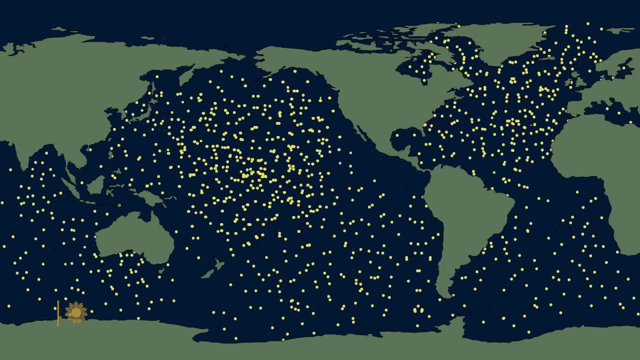 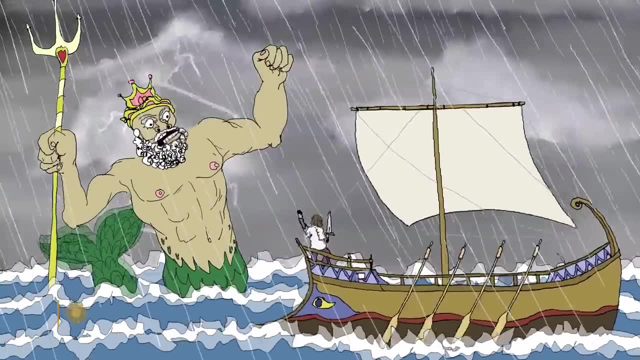 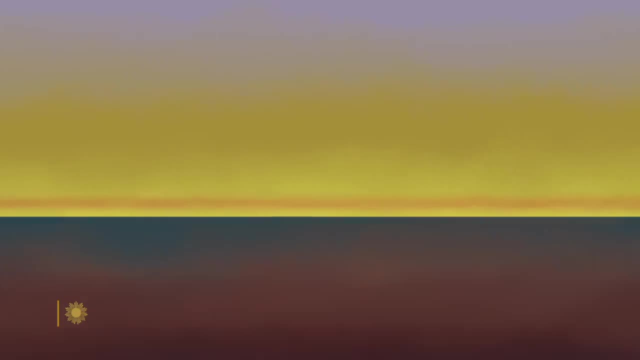 are more than 3,000 of them now in the oceans, more all the time. they're called Argos, after Jason and the Argonauts in Greek mythology, and, combined with various other measuring projects, they tell us that oceans are getting warmer. the upper 700 feet have already warmed by 1.3 degrees Fahrenheit since 1900. now, 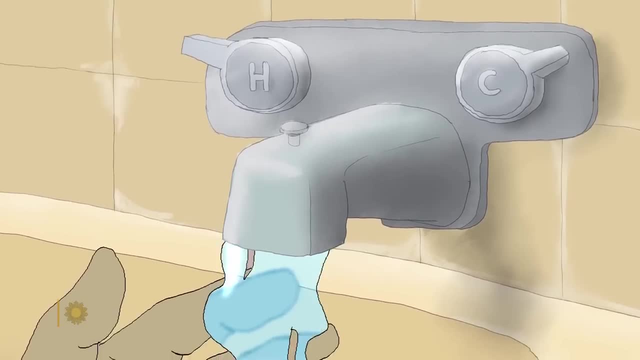 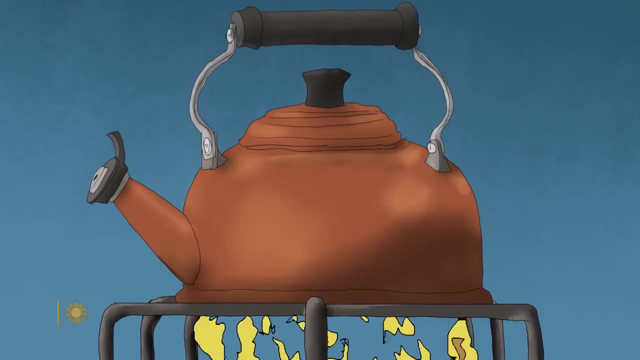 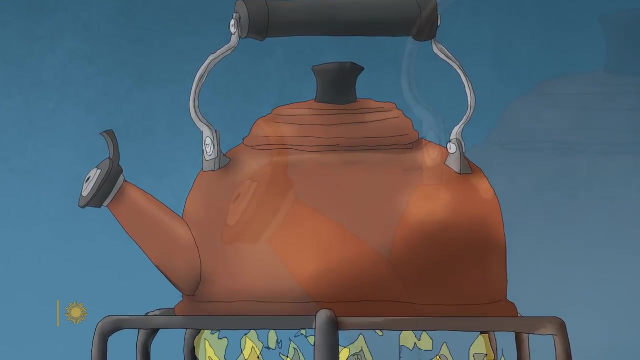 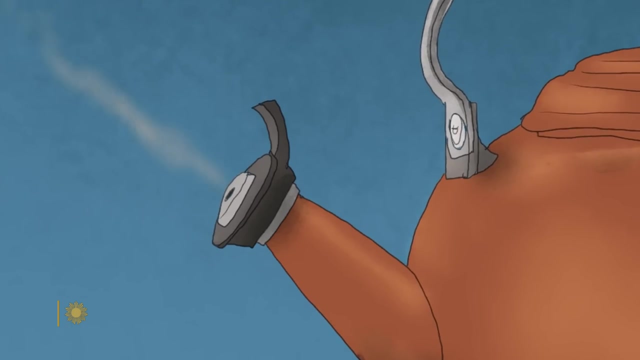 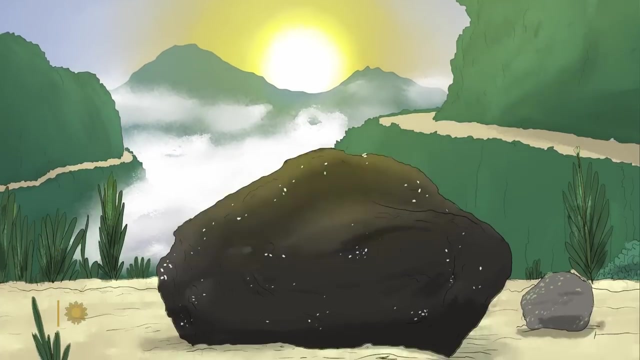 if 1.3 degrees seems like, yeah, come on, that's nothing. remember how long it takes to warm a pot of tea. I mean it can take. well, water has what scientists call a high heat capacity, which means on a sunny day it's a dark stone will get very hot almost immediately. same with the hood of a 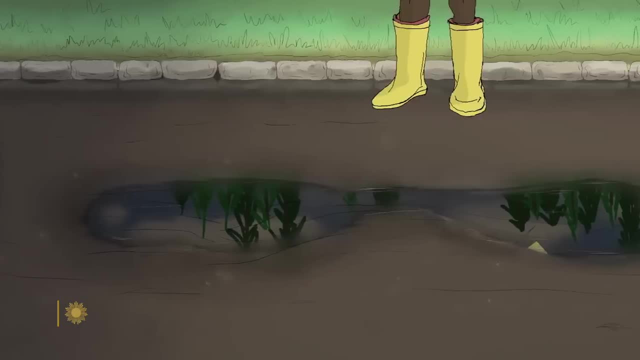 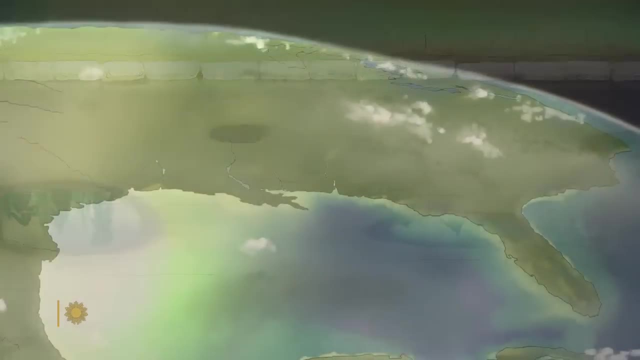 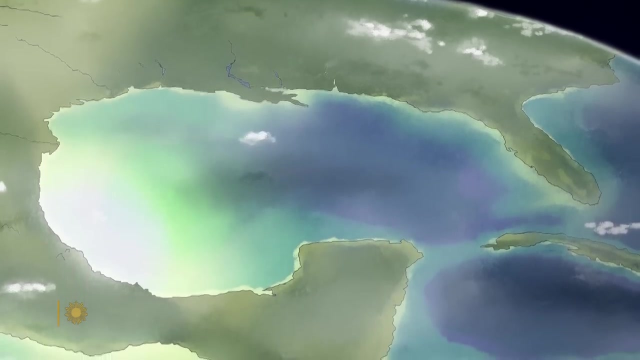 black car. but a puddle of water takes more time and needs more sunshine to get even one degree warmer. so it's kind of a surprise that the surface of an enormous puddle- quadrillions of tons of ocean water- has already warmed by more than a degree. now the oceans don't look different, but it turns out each extra.